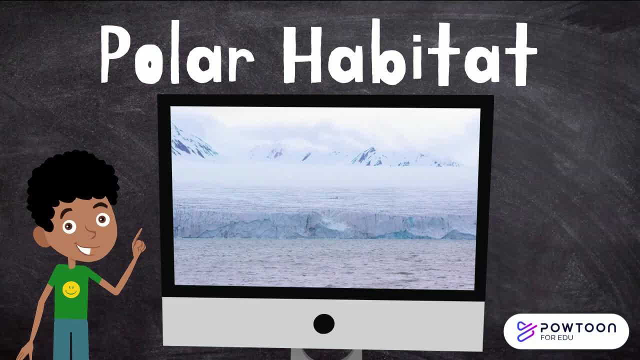 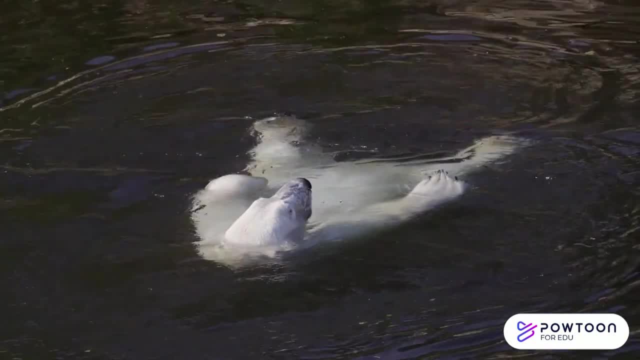 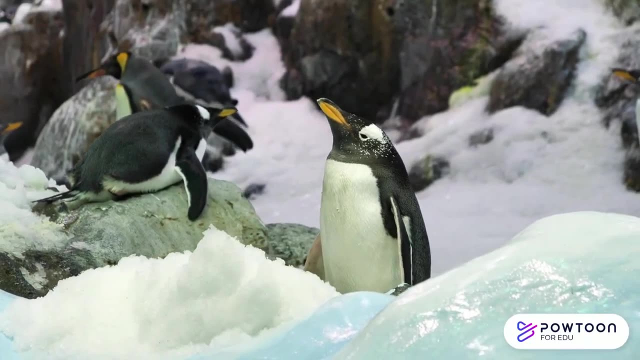 to have extra fur and body fat to survive the cold weather. Some of the animals found in polar habitats are polar bears, snowy owls and penguins. Most of the animals are carnivores here, as they can't rely too much on eating plants. 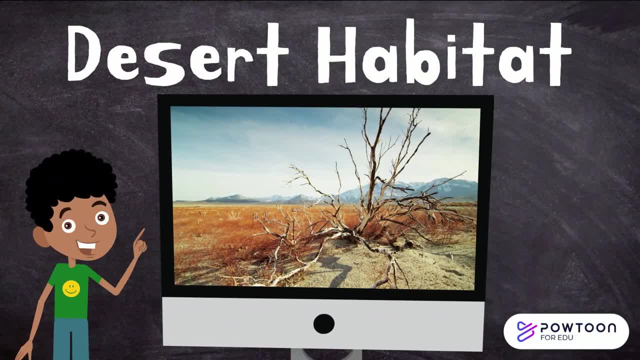 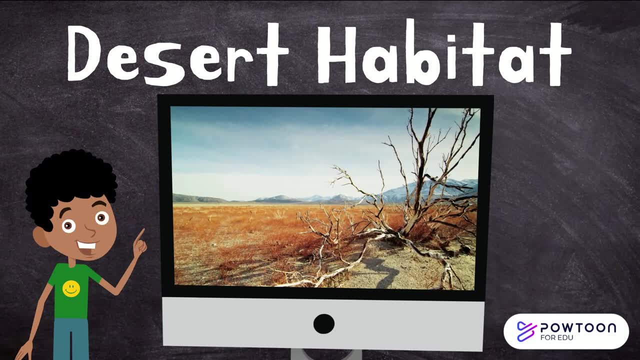 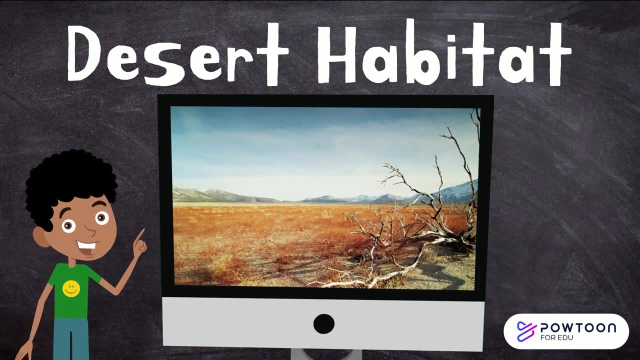 Now we're going to look at the desert habitat. This is very dry and gets very little rain. Animals and plants have adapted to survive these harsh conditions and to survive without much water. Cactus have sharp spines and needles to help protect them from animals. 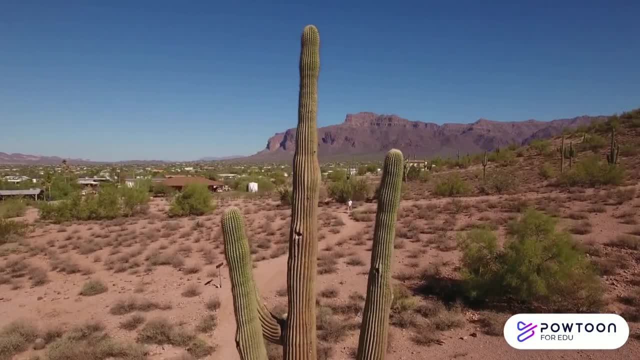 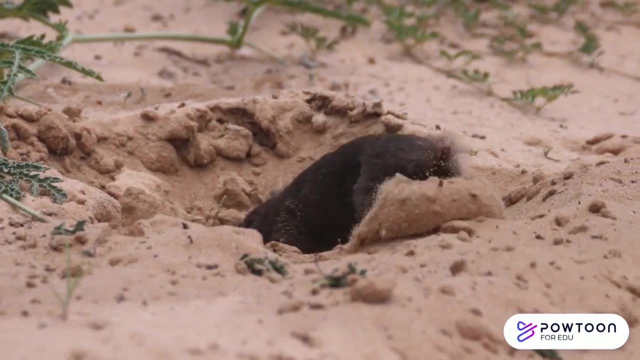 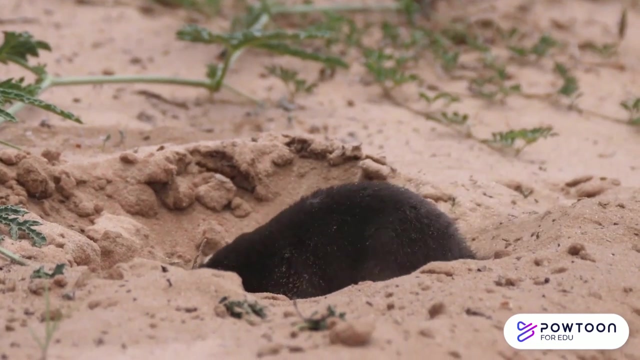 and are able to store water in their roots and trunks to survive a long time without rain. Most desert animals stay underground or beneath shady rocks during the day. Many of them come out to hunt for food at night, when it's cool. Some of the animals you'll 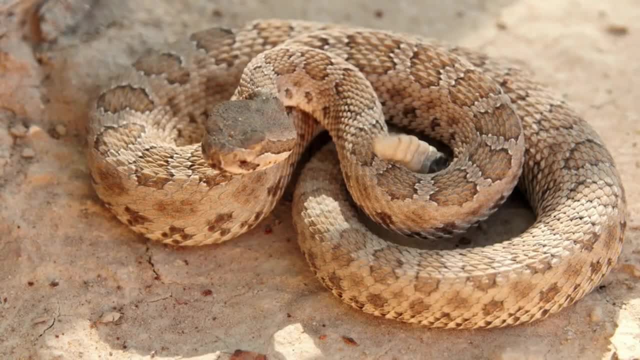 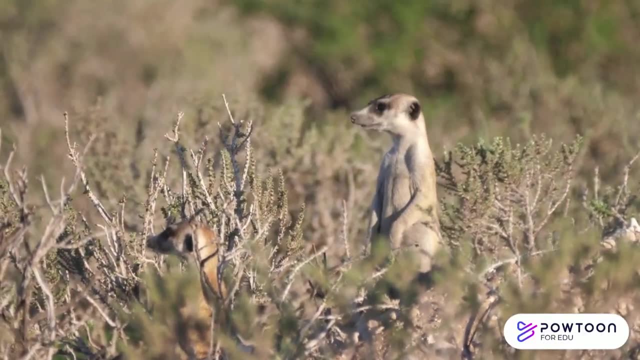 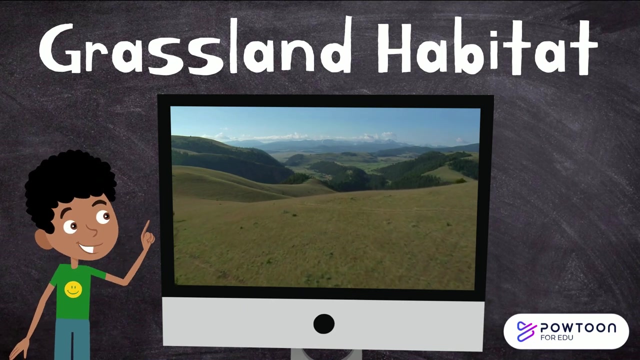 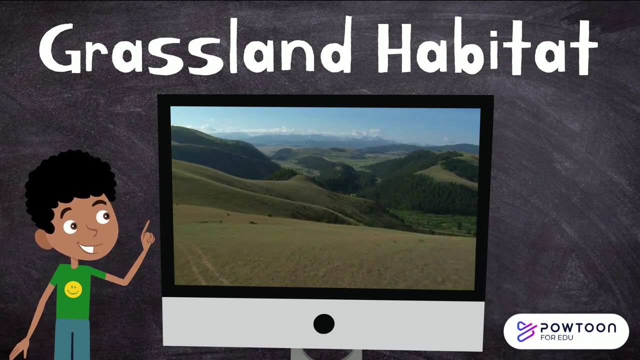 find in this habitat are snakes, meerkats and fennec foxes. Now let's look at grassland habitats. These habitats are large spaces with various grasses and fewer trees. The amount of rain is not enough to grow tall trees and produce. 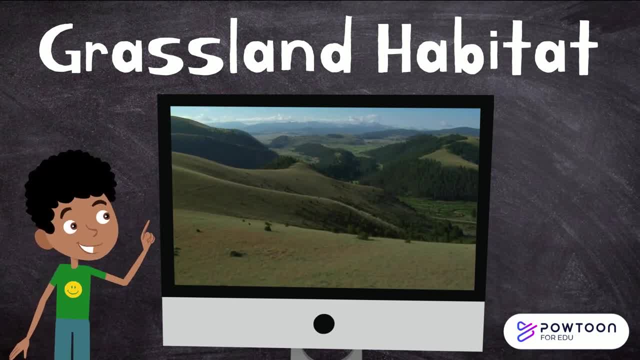 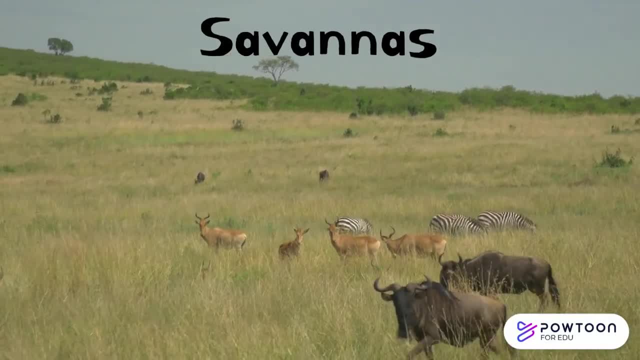 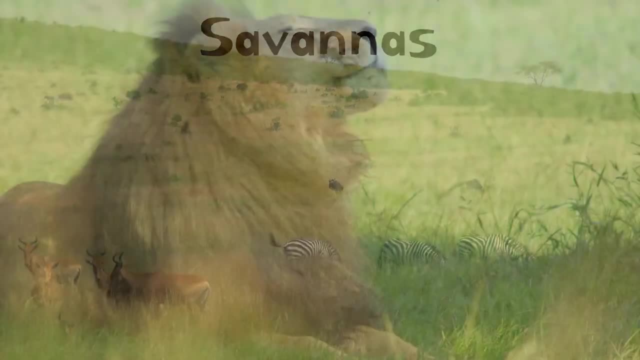 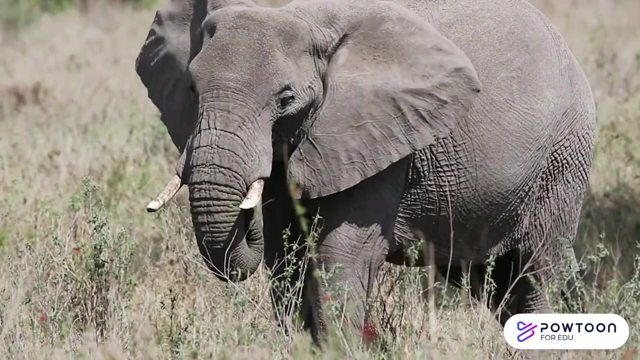 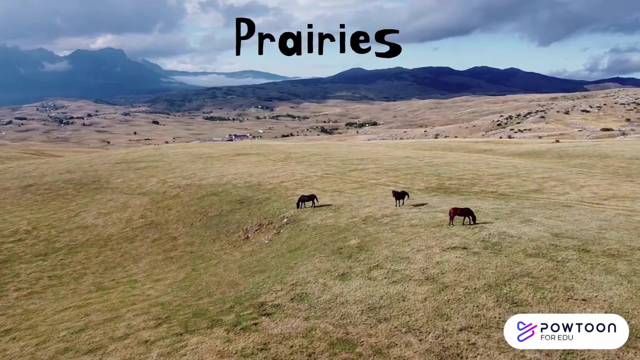 a forest, but is enough for it not to be a desert. There are different types of grasslands found on different continents. The grasslands found in Africa are called savannas. Here you'll find lions, elephants and giraffe. The grasslands in North America: 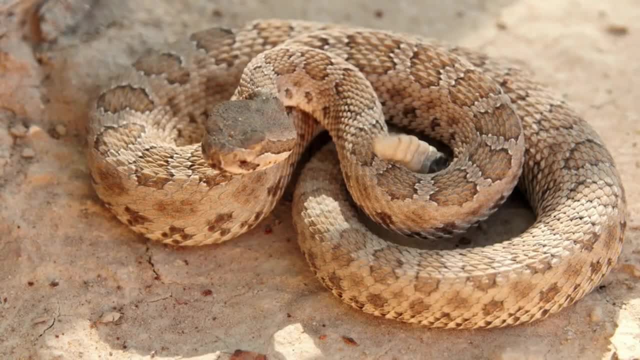 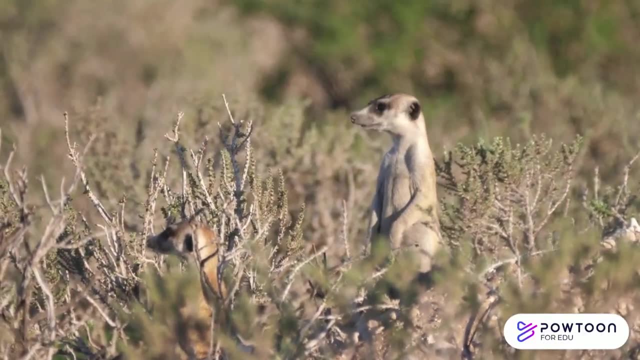 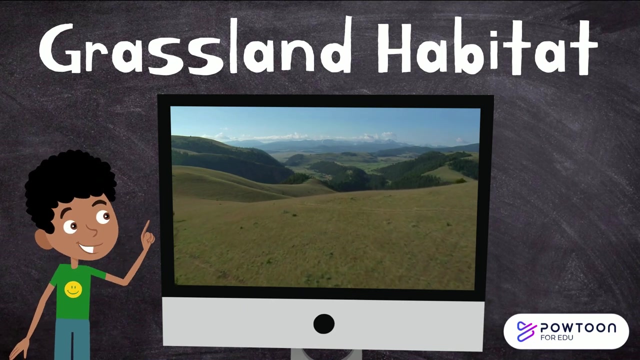 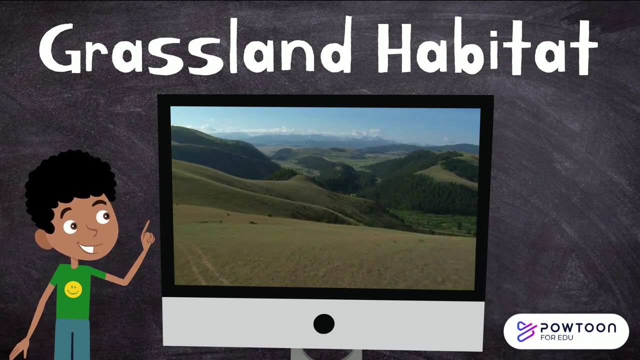 find in this habitat are snakes, meerkats and fennec foxes. Now let's look at grassland habitats. These habitats are large spaces with various grasses and fewer trees. The amount of rain is not enough to grow tall trees and produce. 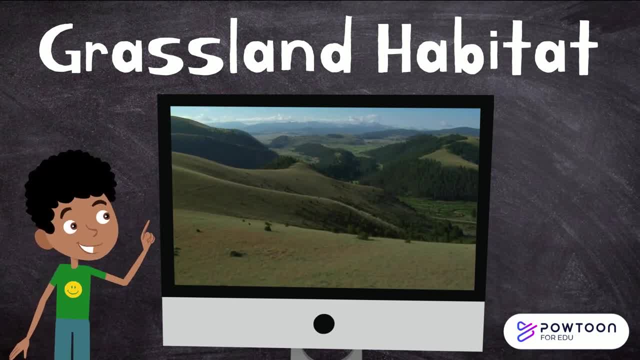 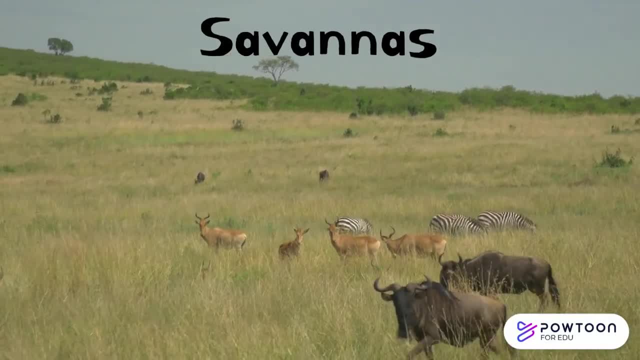 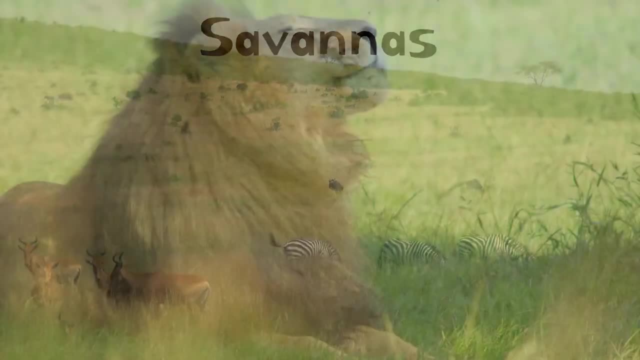 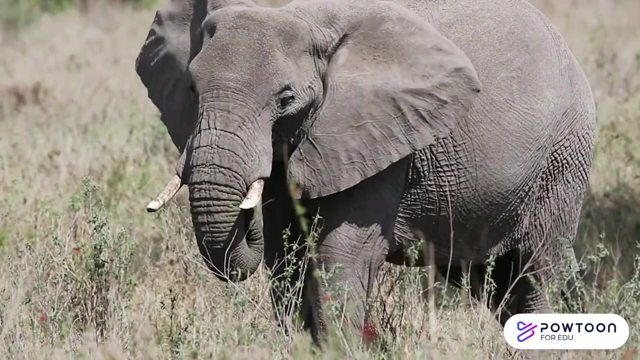 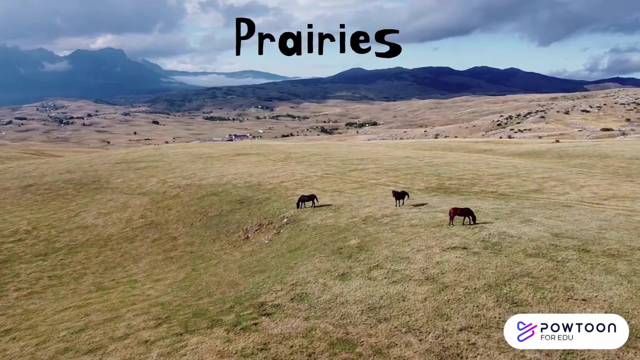 a forest, but is enough for it not to be a desert. There are different types of grasslands found on different continents. The grasslands found in Africa are called savannas. Here you'll find lions, elephants and giraffe. The grasslands in North America: 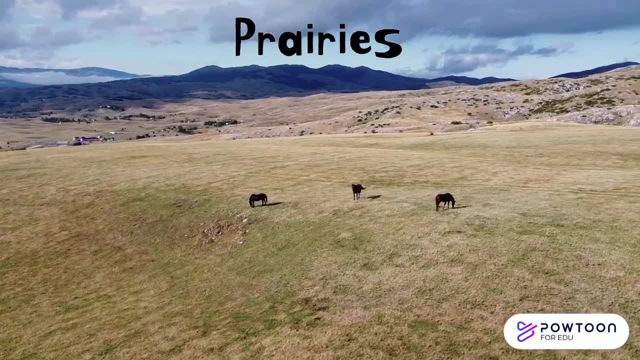 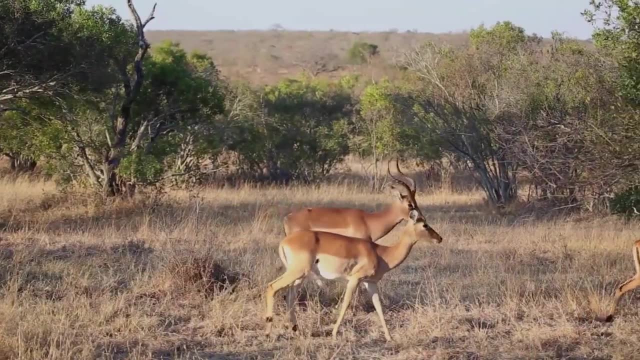 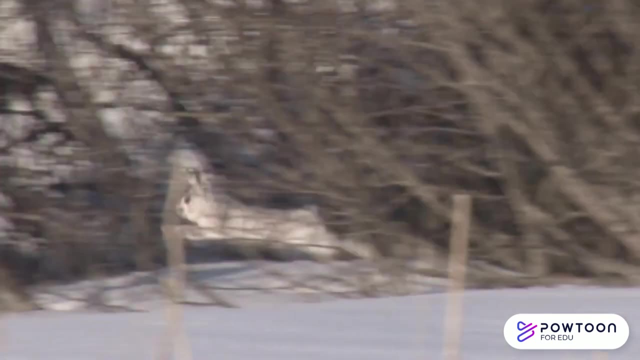 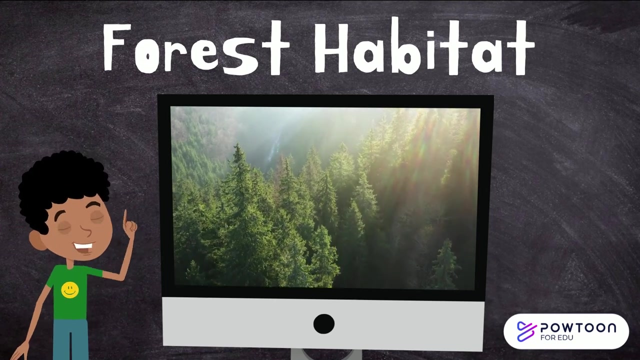 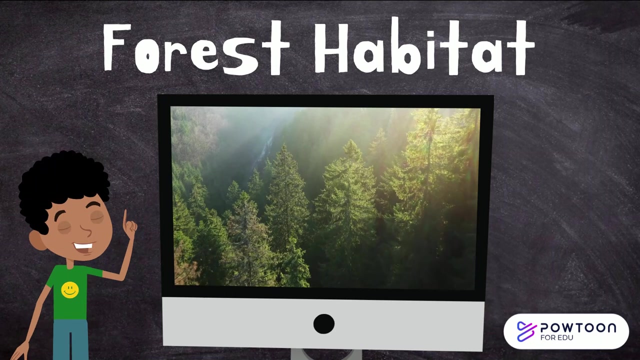 are called prairies. Here you'll find coyotes, antelope and rabbits. Next, let's look at forest habitats. These habitats have various types of trees. Many birds and animals live within this habitat. There are three types of forest. 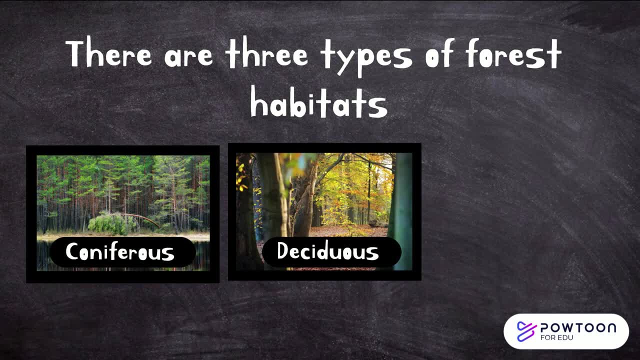 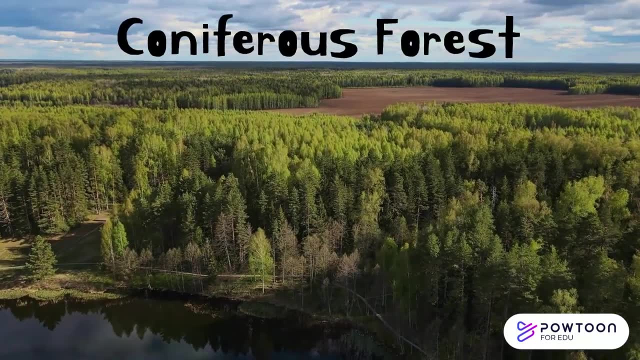 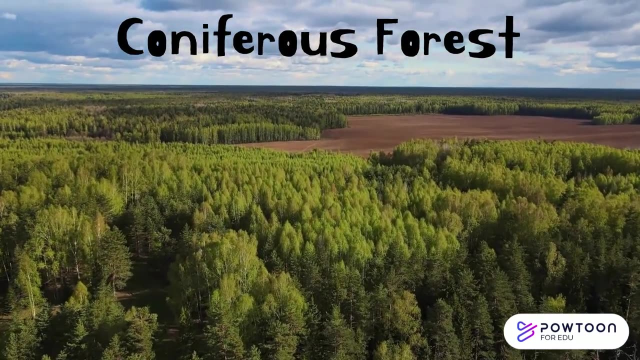 habitats: Coniferous, deciduous and rainforest Coniferous forests. The main trees here are evergreen conifers, which produce seeds in cones. There are not many different types of trees in coniferous forests because of the cold weather. 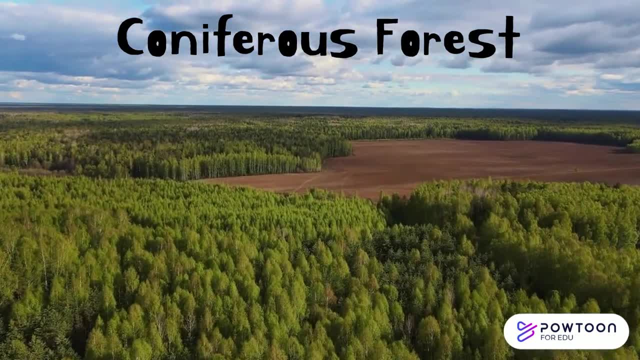 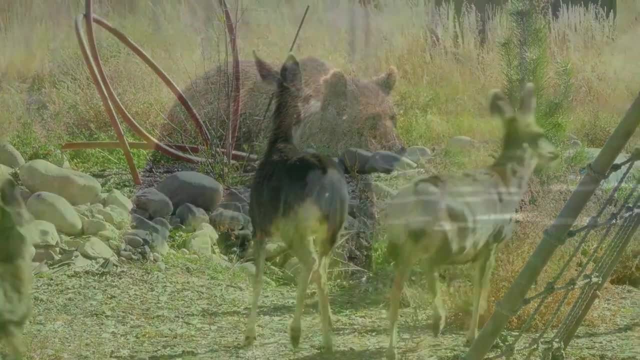 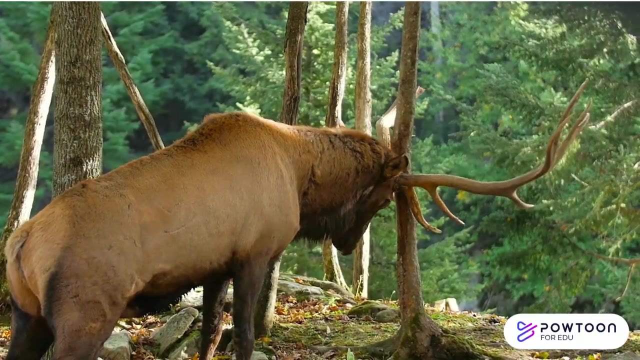 and the poor soil. Some animals that live in coniferous forests are deers, bears and caribou. Some animals that live in coniferous forests are deers, bears and caribou Deciduous, also known as. temperate forests mostly grow in North America, Europe and Asia. They have a moderate climate and experience the spring, summer, fall and winter. During winter, many animals migrate or hibernate. Animals that we may see in this habitat include bears, raccoons and squirrels. 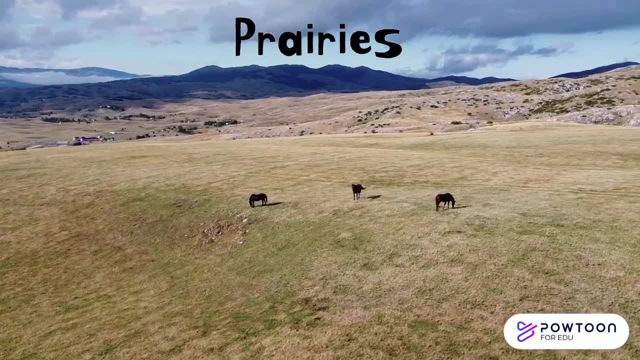 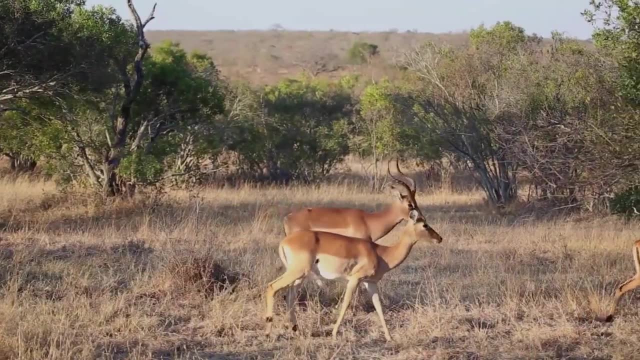 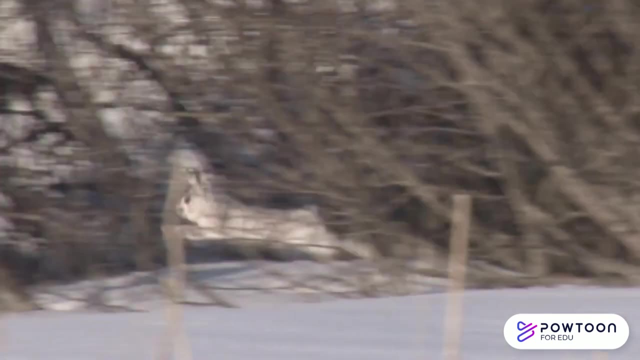 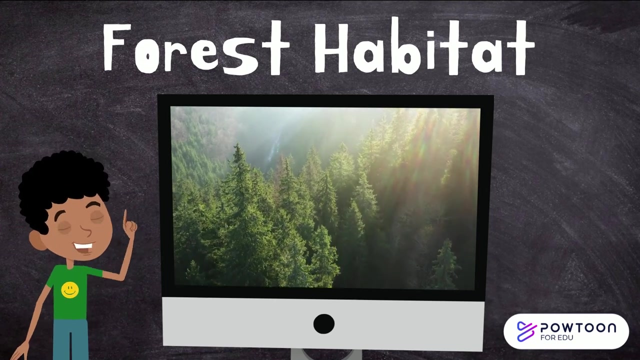 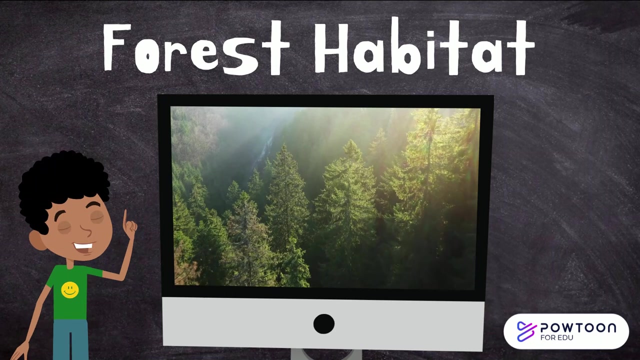 are called prairies. Here you'll find coyotes, antelope and rabbits. Next, let's look at forest habitats. These habitats have various types of trees. Many birds and animals live within this habitat. There are three types of forest. 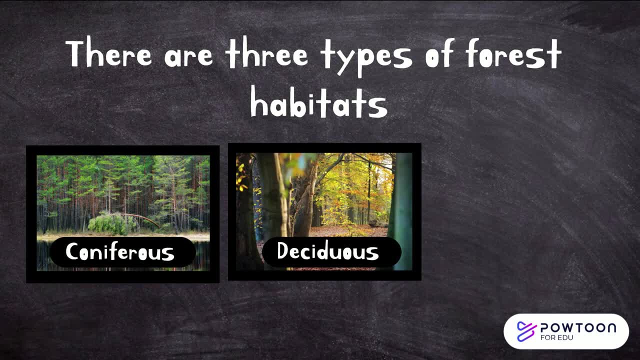 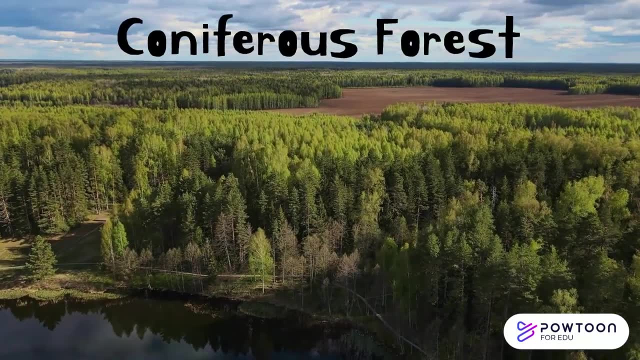 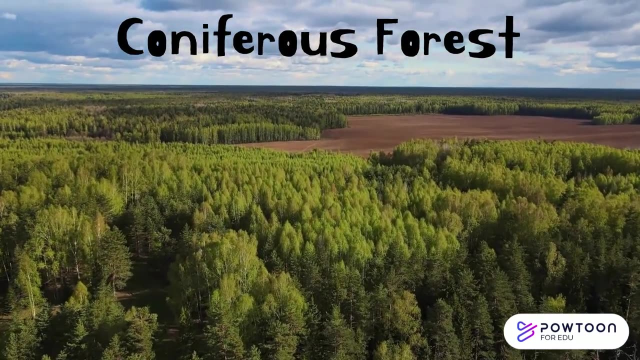 habitats: Coniferous, deciduous and rainforest Coniferous forests. The main trees here are evergreen conifers, which produce seeds in cones. There are not many different types of trees in coniferous forests because of the cold weather. 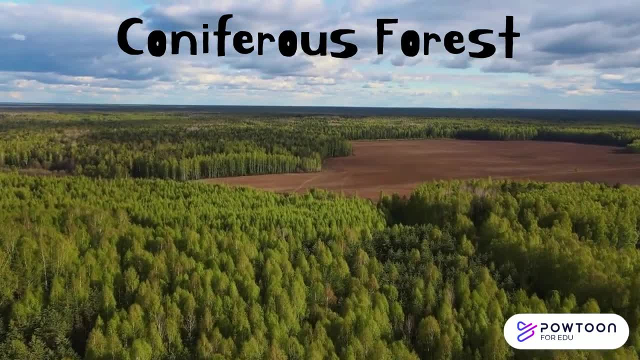 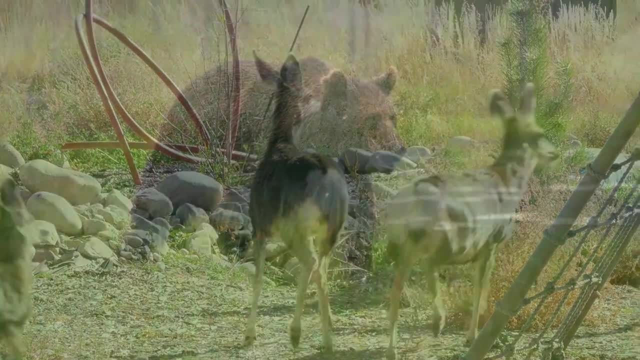 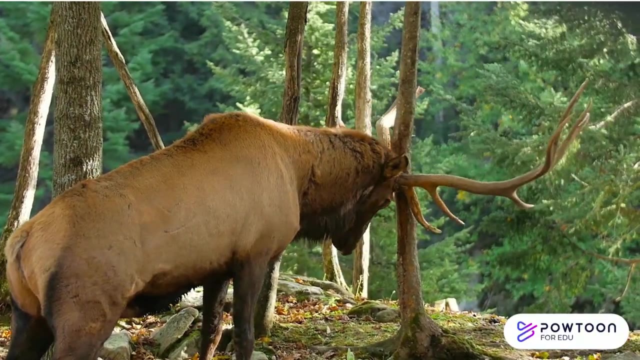 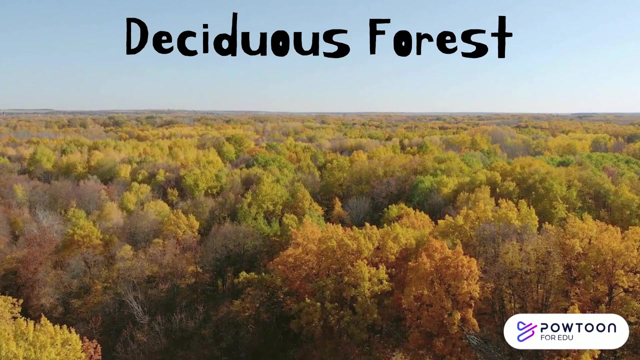 and the poor soil. Some animals that live in coniferous forests are deers bears and caribou Deer bears and caribou Deer bears and caribou Deciduous, also known as temperate. forests mostly grow in North America, Europe and Asia. They have a moderate climate and experience the spring, summer, fall and winter. During winter or hibernate, Animals that we may see in this habitat include bears, raccoons and squirrels. 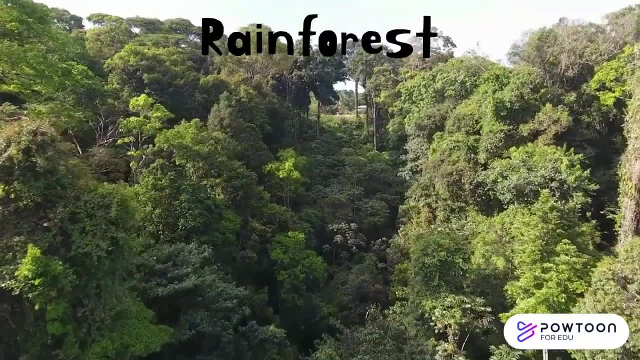 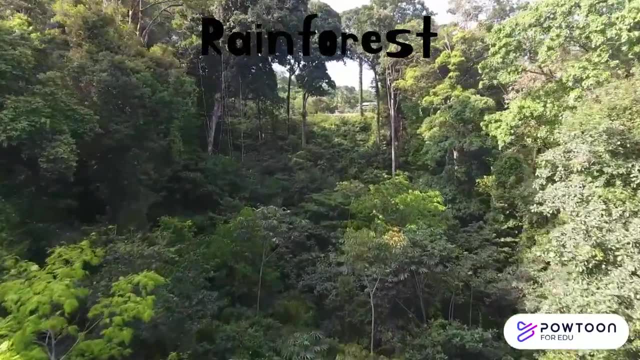 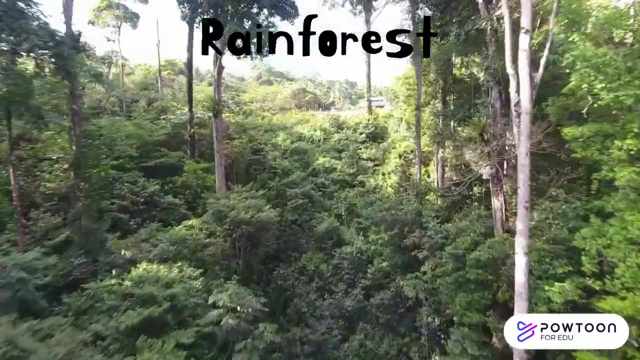 Rainforests, If the name doesn't already give you a clue. well, it rains a lot in this habitat. It is much wetter and hotter than the other forests. Rainforests have the most amount of diverse plants and animals than any other habitat. Some animals that you will find here are: 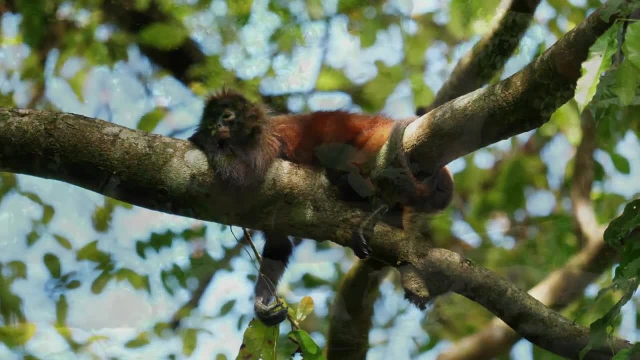 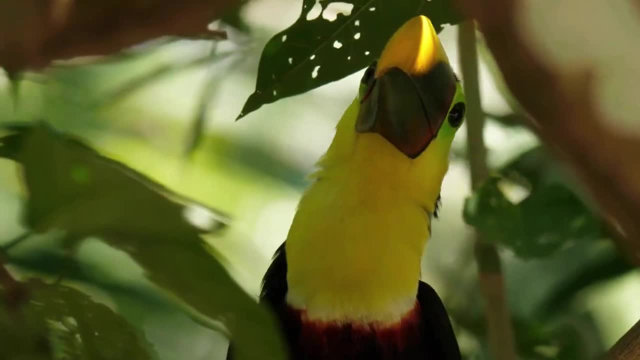 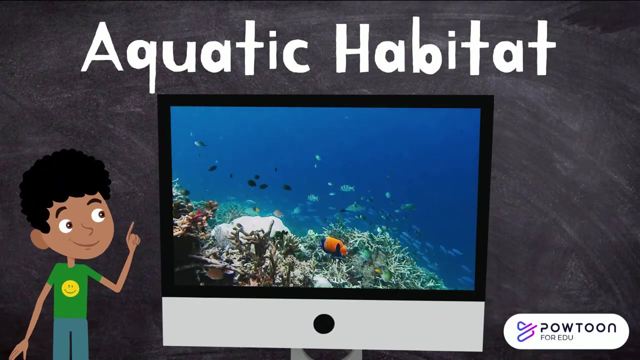 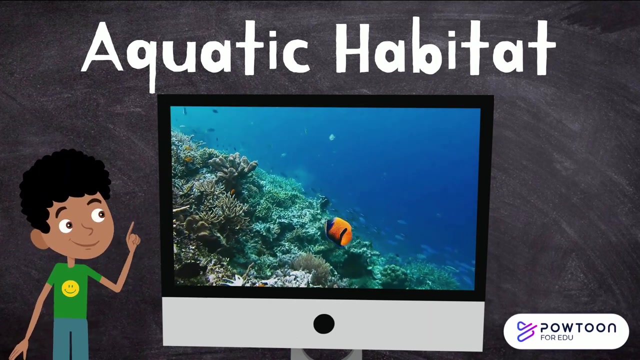 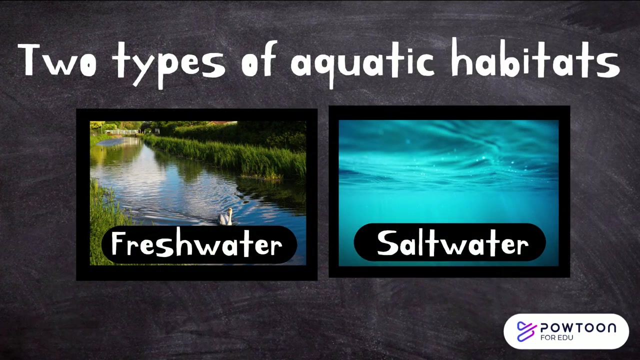 monkeys, jaguars and many bright and colorful birds like toucan. The final habitat we're going to look at today is water, or aquatic habitats. Now, this covers most of the earth's surface and can be split up into two types: Freshwater habitats and saltwater habitats. 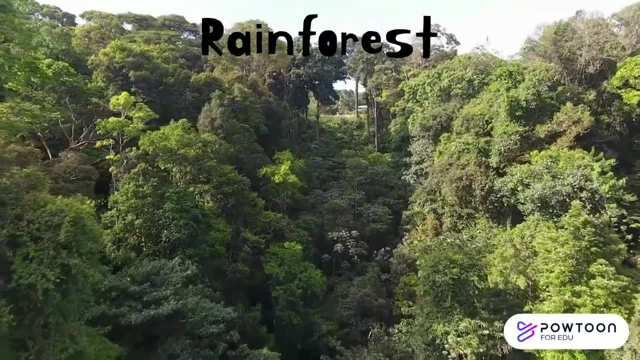 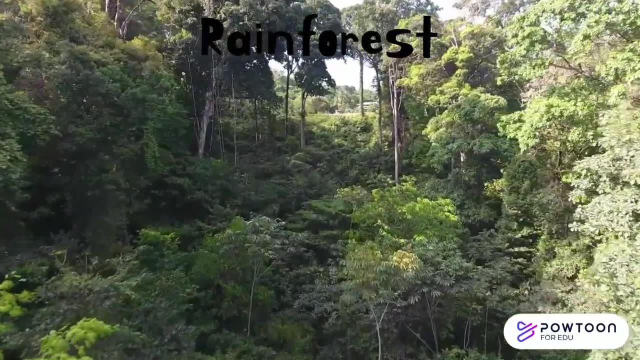 Rainforests, If the name doesn't already give you a clue. well, it rains a lot in this habitat. It is much wetter and hotter than the other forests. Rainforests have the most amount of diverse plants and animals than any other habitat. 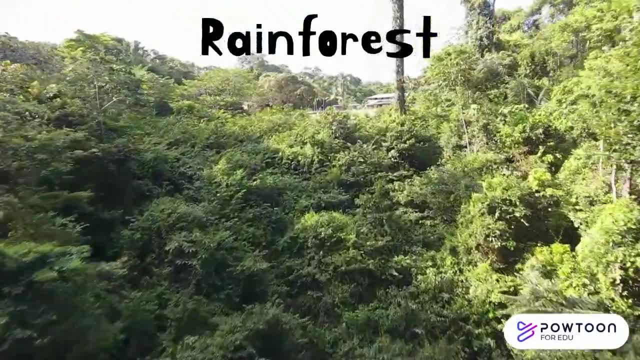 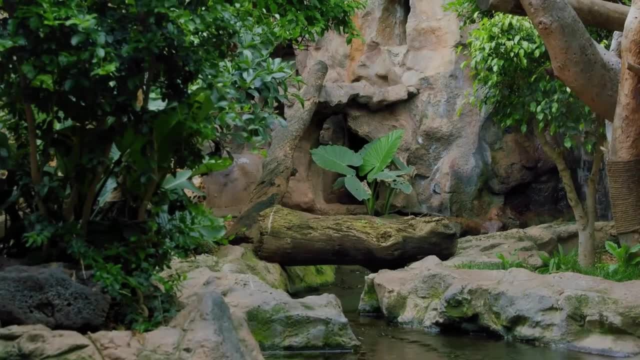 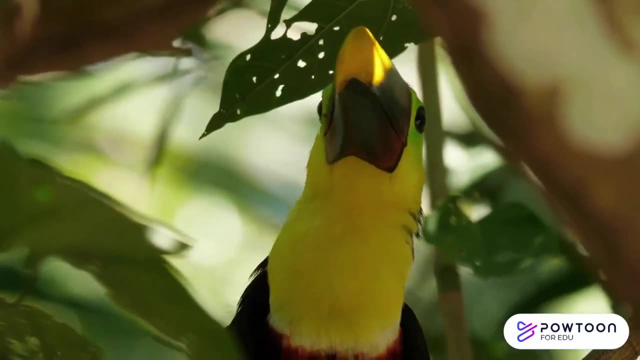 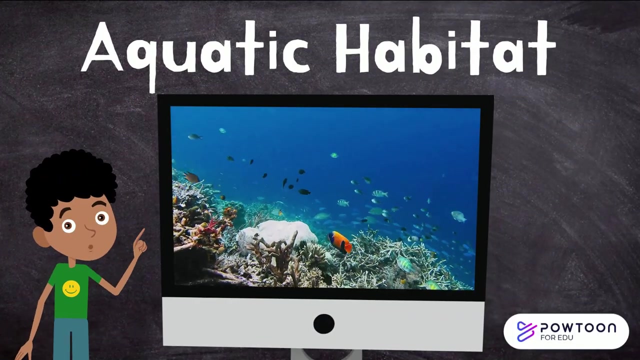 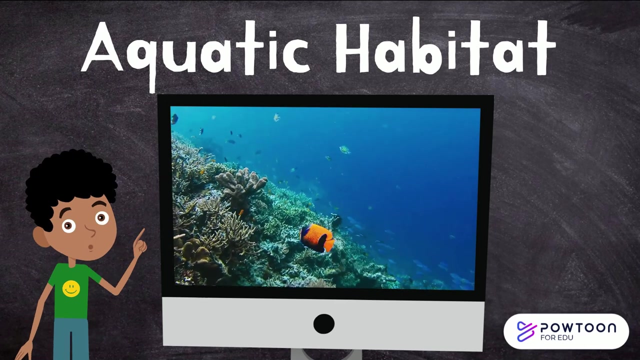 Some animals that you will find here are monkeys, jaguars and many bright and colourful birds Like the toucan. The final habitat we're going to look at today is water, or aquatic habitats. Now, this covers most of the earth's surface and can be split up into two types. 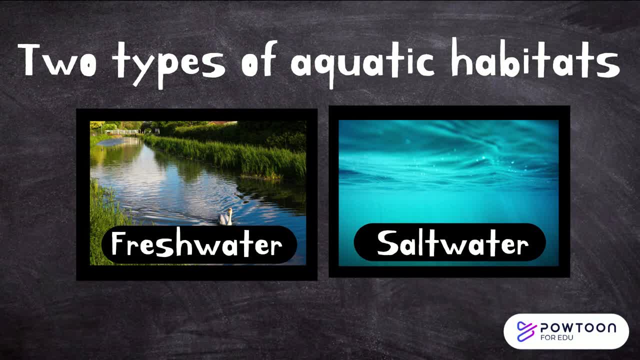 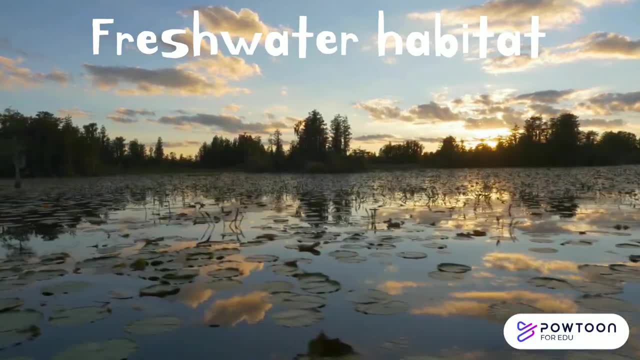 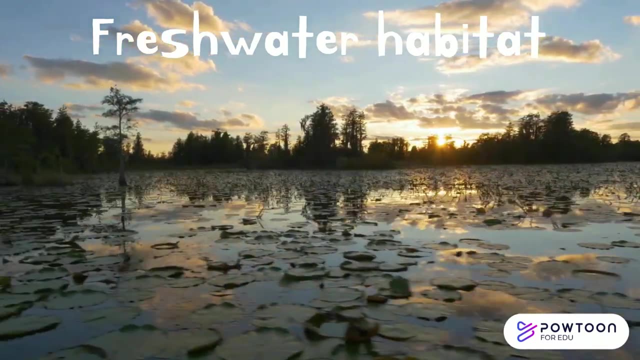 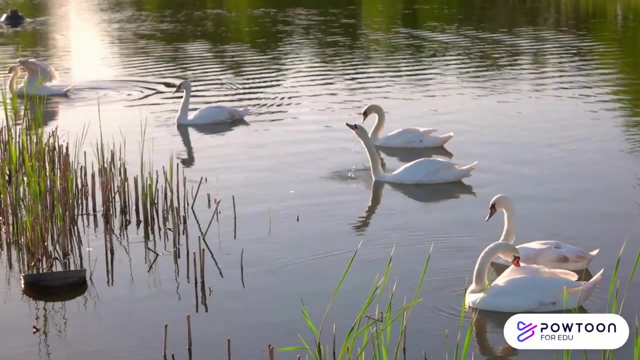 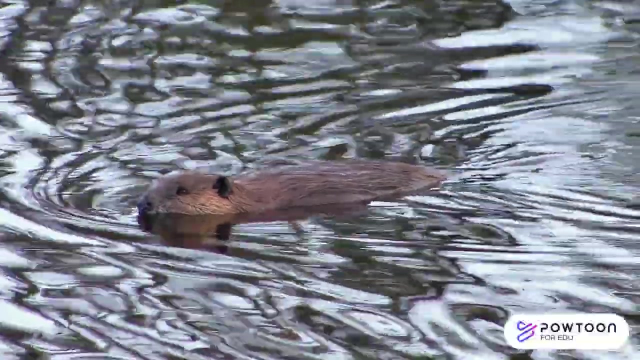 Freshwater habitats and saltwater habitats. Freshwater habitats are bodies of water that have very low soil density. they all contain very low amount of salt. These include bodies of water such as swamps, lakes and ponds, Frogs, beavers. 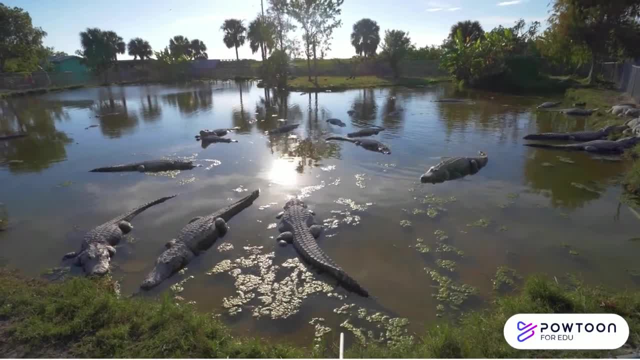 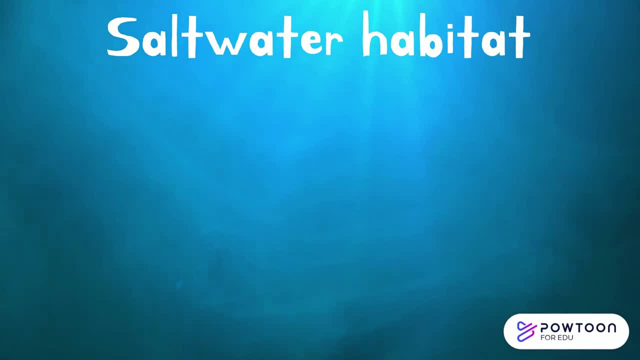 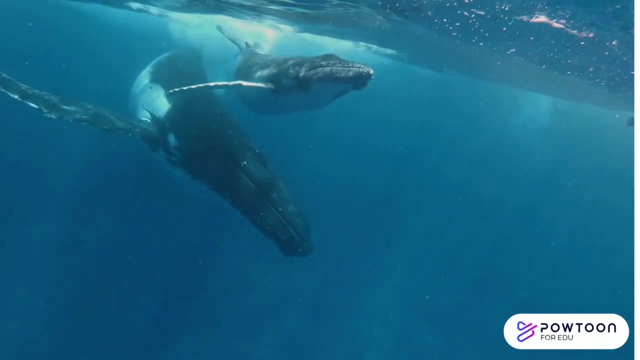 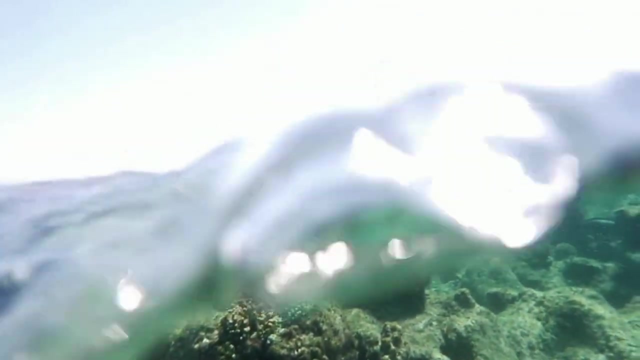 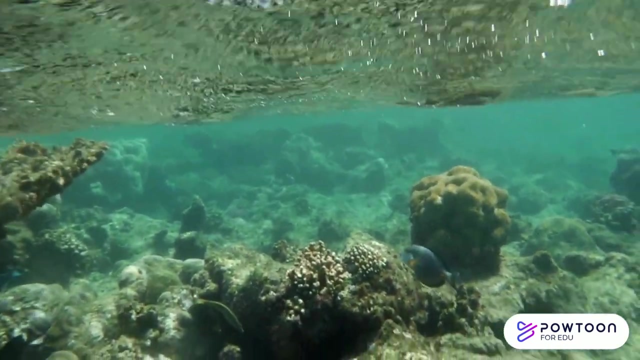 and alligators All live in freshwater habitats. Saltwater or ocean habitats covers over 70% of the Earth's surface and includes open oceans where many marine animals live, such as sharks, whales and dolphins. Coral reefs are also a saltwater habitat. They grow slowly in warm, shallow tropical waters, building up their colourful shapes over hundreds and thousands of years. 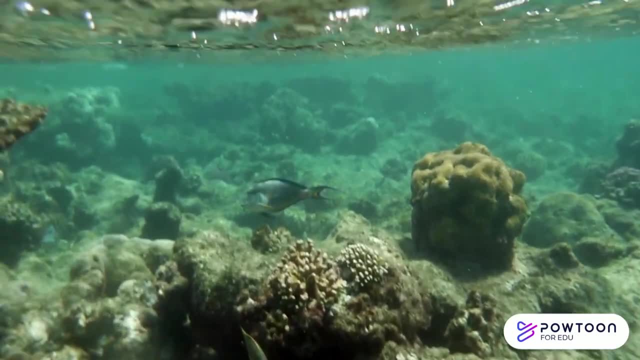 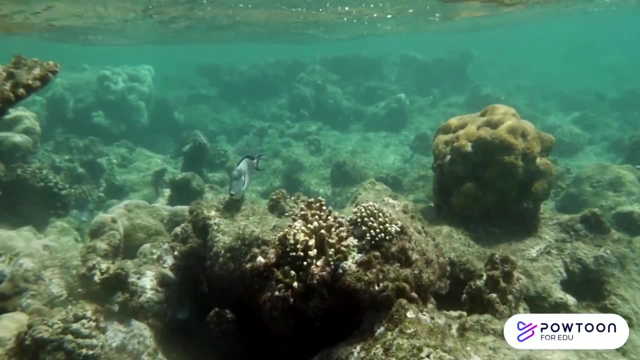 Coral reefs are one of Earth's most diverse habitats, with creatures such as fish, corals, lobsters, clams, seahorses, sponges and sea turtles calling this their home. Thank you for learning all about the coral reef. 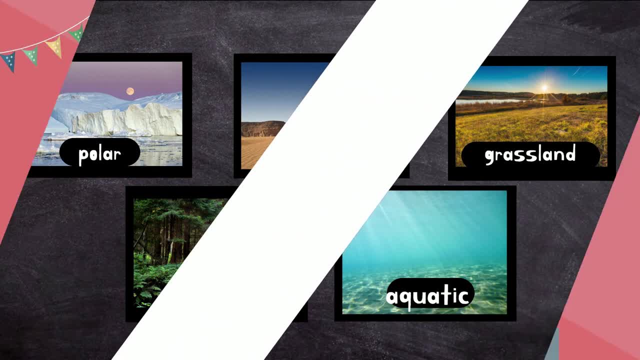 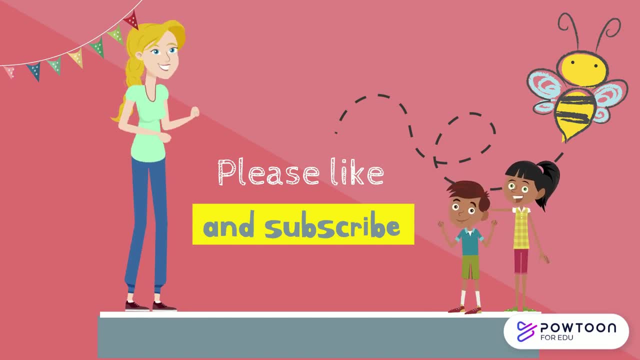 Thanks for watching. If you like this video, please like and subscribe, and don't forget to check out the other videos on Buzz with Bea.